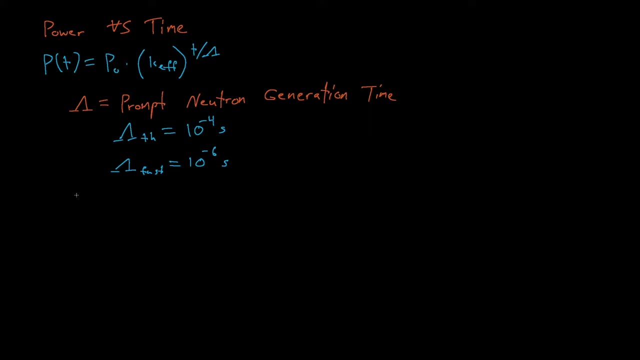 through the chain reaction chain. If K effective is greater than 1, then each step in our chain reaction will on average generate more neutrons and increase the power of our system. So let's say we insert a small 20-cent reactivity insertion into our system. We'll discuss what cents and dollars. 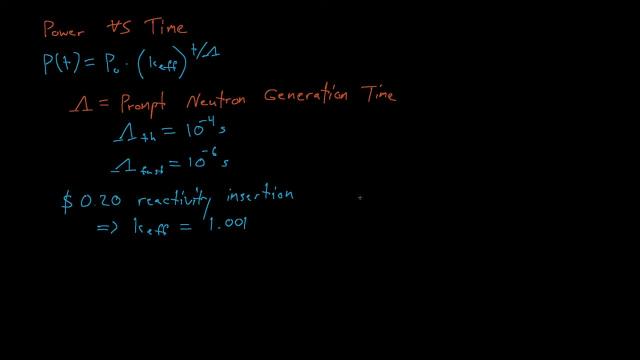 mean later, but for now just know that this is a relatively minor change in our system. This reactivity change will cause the reactor power to increase because the system is now stable. Let's say that our reactor operator wants to keep things critical and responds as fast as they can by inserting the control rods. Now the 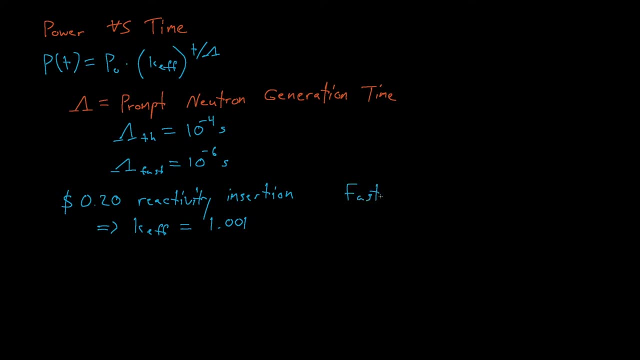 average human reaction time is about 0.25 seconds and the fastest human reaction time pretty much ever recorded is 0.101 seconds. So let's say that our reactor operator is the Usain Bolt of reactors, the Hungrybox or the Michael. 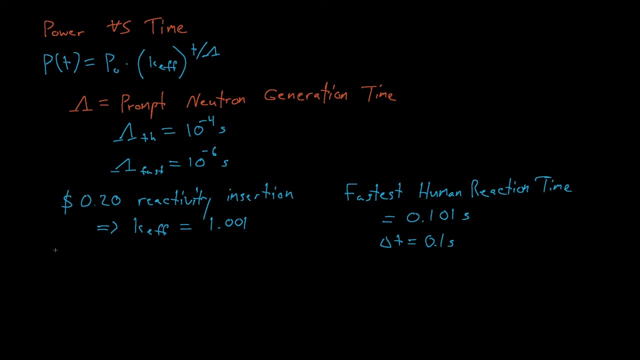 Jordan of reactors so they can respond actually in about 0.1 seconds. In that time the reactor power will have increased by 172 percent for a thermal reactor and it will have increased by a factor of 2.557 times 10 to the 43 for a 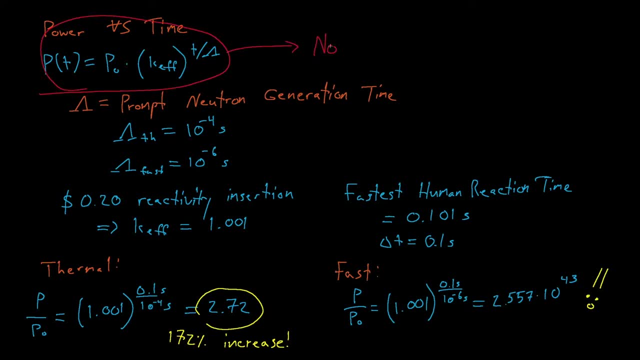 fast reactor. Clearly this model is not realistic. Thermal reactors operate all the time without having such huge destabilizing power swings, and we've actually operated fast reactors at steady state without blowing up the universe. So why is our naive model incorrect? Our model is wrong for two. 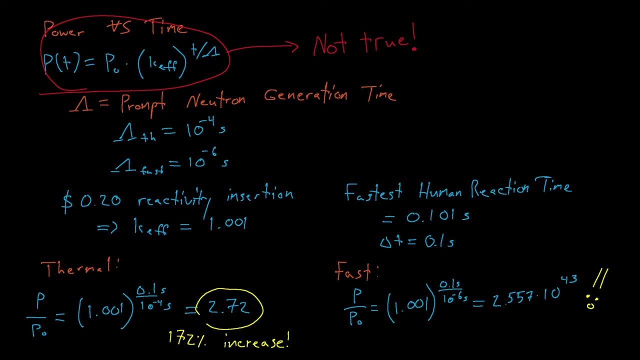 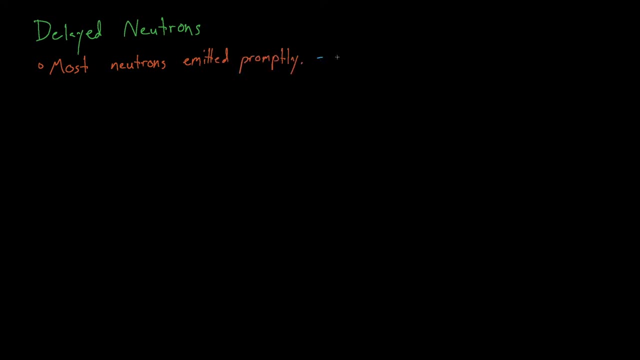 reasons: Delayed neutrons and feedback. Let's talk about delayed neutrons. Most of the neutrons in a reactor are emitted promptly, which means that they're emitted about 10 to the negative 14 seconds after a fission occurs, But less. 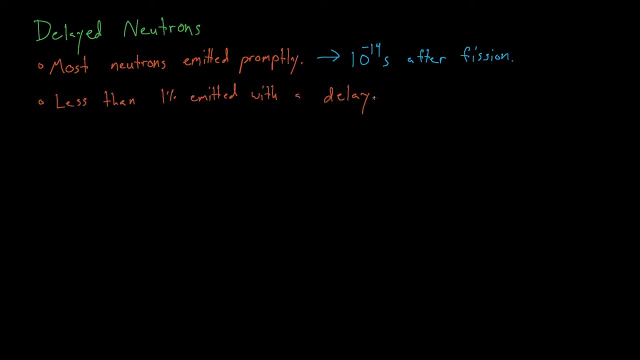 than about 1% of neutrons are emitted with a delay on the order of 0.1 to 1.0 seconds. These neutrons are known as delayed fission neutrons, and they're actually not emitted from fission. despite their name, They're actually emitted by fission. 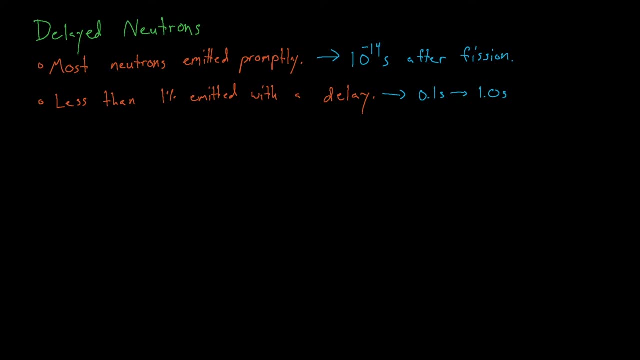 products as they begin to undergo radioactive decay. These fission products are neutron rich, so they tend to decay by emitting neutrons. The variable beta or beta-effective is known as the delayed neutron fraction and, as its name suggests, it is just the fraction of neutrons emitted from fission in our system that are 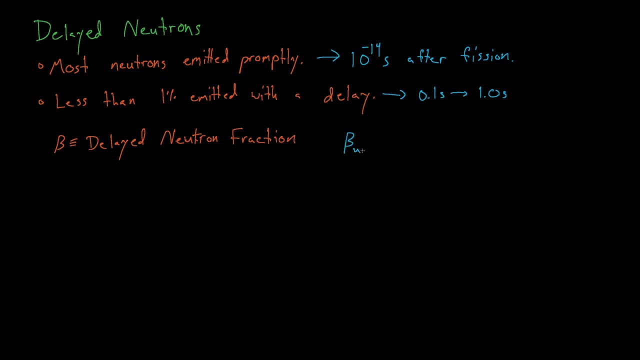 emitted by these delayed neutron precursors. Beta is about 0.0065 for uranium-235 and about 0.0020 for plutonium-239,, meaning that plutonium releases fewer delayed neutrons and actually is more difficult to control than a uranium reactor. These delayed neutron fractions might not sound. 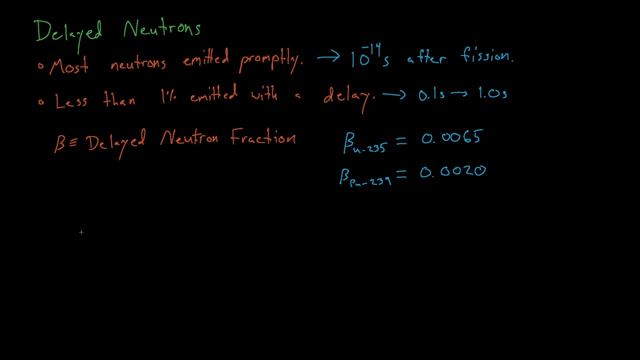 very significant, but they're actually significant enough for us to control a reactor. All reactors are operated so that they're actually subcritical. if you only consider prompt neutrons, They must have delayed neutrons to be able to maintain a critical chain reaction. This means that power 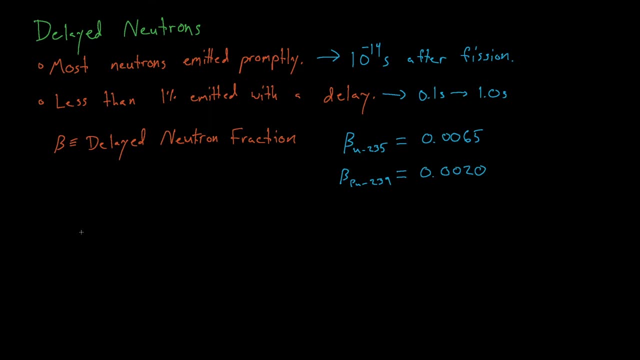 increases in a reactor are really constrained by the time scale on which delayed neutrons are emitted, which is seconds to tenths of seconds, not nanoseconds like prompt neutrons. This really slows things down. It makes our reactors very controllable. Now, when a reactor's K-effective exceeds 1, plus its 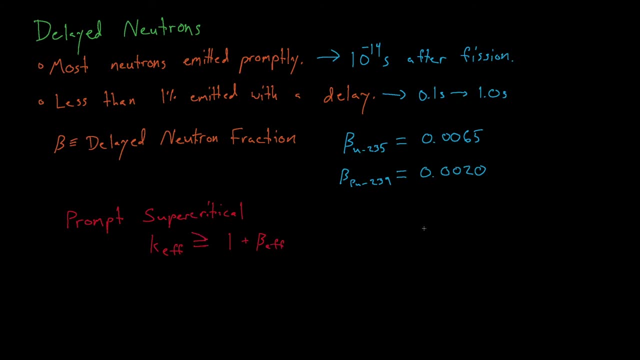 beta-effective value. it is now supercritical, using only prompt neutrons, which means that its power goes back to increasing exponentially at a mind-blowing and possibly reactor-blowing rate. Now, another key concept in kinetics is the reactivity of a system. Reactivity simply measures. 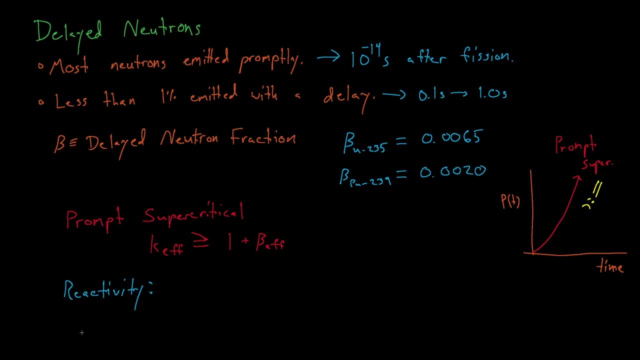 how far a reactor is above or below the reactor's k-effective value. When a reactor's k-effective is above or below being critical- basically how super or subcritical it is- reactivity is just equal to the reactor's k-effective minus 1 divided by k. Reactivity is usually expressed in units of. 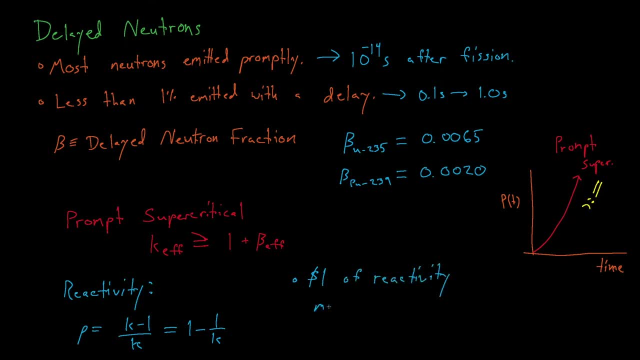 dollars and cents, where one dollar of reactivity means that k-effective is equal to 1 plus beta- effective. Thus one dollar of reactivity will make our reactor enter the dreaded prompt supercritical regime. The term cents is just 1 one-hundredth of a dollar, since there are 100 cents in a dollar. 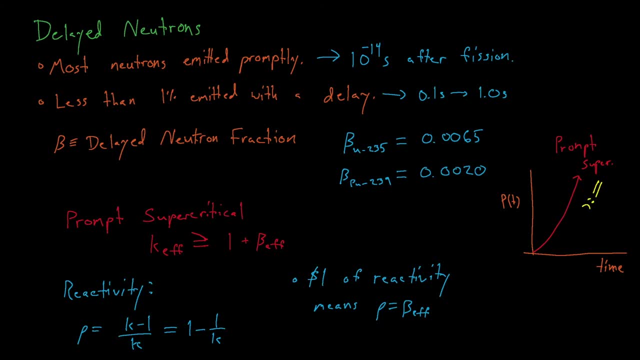 These dollar and cent terms were actually developed by scientists at Los Alamos during the Manhattan Project, Just like the terms barns or shakes. dollars and cents were used so that the scientists could go to bars, restaurants or other public places and keep discussing work as nuclear. 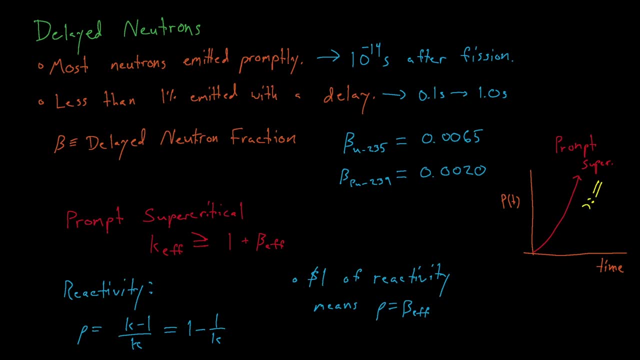 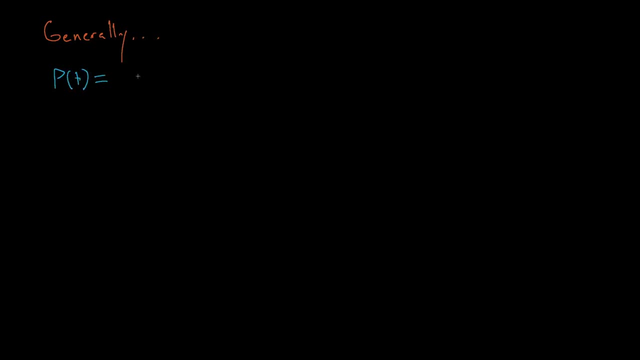 engineers tend to do without revealing classified topics. The power of reactors that are either supercritical or supercritical-but-not-prompt supercritical can be approximated using this equation, where rho is our reactivity from above and the little lambda is the average decay constant. 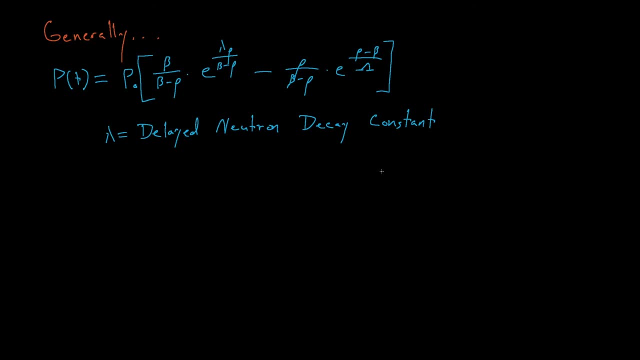 for our delayed neutron emission Because all commercial reactors operate in this regime, except for Chernobyl during its accident. this equation can be used to approximate how a reactor's power will respond to changes or reactivity insertions. Now what happens when things get? 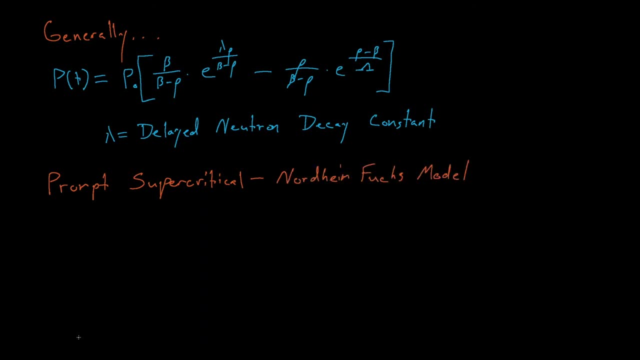 supercritical. The Nordheim-Fuchs model is a relatively simple yet fairly effective way for predicting a reactor's power during a prompt supercritical excursion. During this kind of excursion, a reactor's power will increase exponentially at first and then eventually level off and then start to decrease. The shape of this power curve is fairly Gaussian-like. 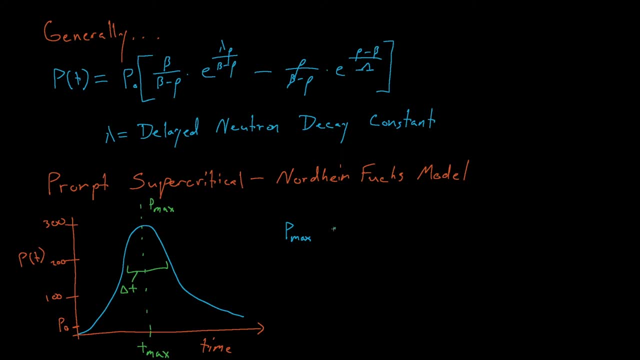 The maximum power that a reactor sees during this excursion is actually inversely proportional to the prompt neutron lifetime, and the width of the peak in time is actually directly proportional to lambda. So why does our power actually peak and then start dropping off instead of increasing forever and ever and causing the next big bang? Well, the power peaks and 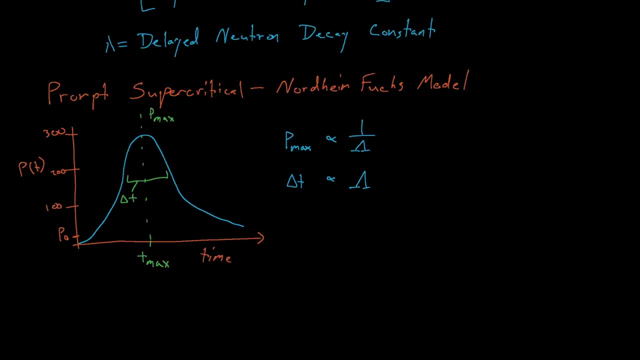 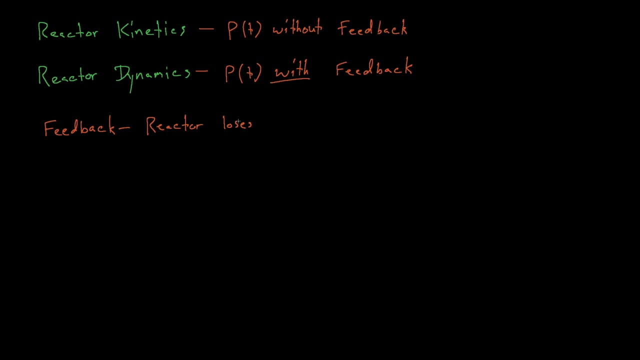 eventually lowers because of something known as feedback. In general, reactor kinetics describes a system's time-dependent behavior without feedback, and reactor dynamics describes this time-dependent behavior with feedback. Feedback refers to the set of phenomena that cause a reactor to become less reactive as its power increases and as it heats up The mechanisms. 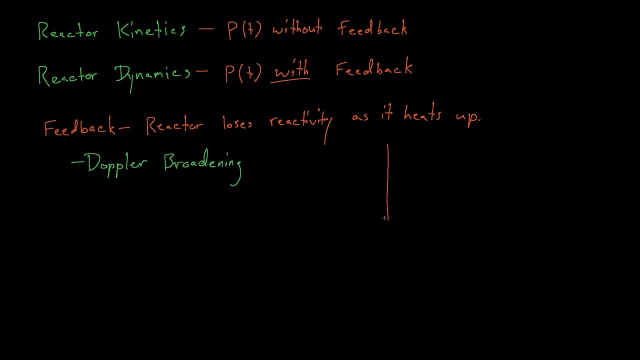 for feedback include Doppler broadening, which we have already discussed to an extent, and some other mechanisms, include a loss of moderation because the moderator either becomes less dense as it heats up or even because it boils away, and also fuel expansion. For fuel expansion.